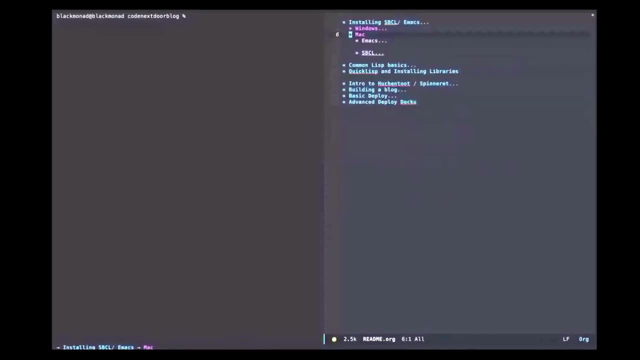 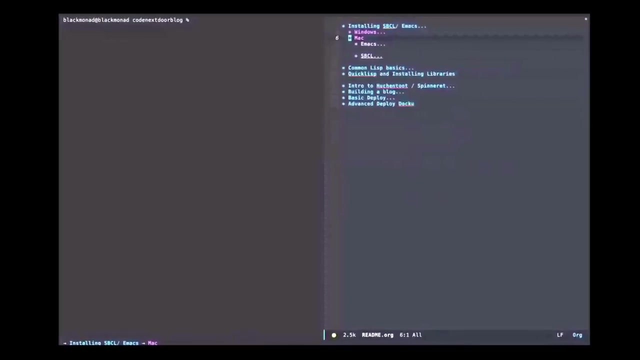 be working with today falls under Common LISP and we will be installing SPCL. If you're running on a Mac machine, I'd say the easiest way to get this is by doing brew install SPCL. if you don't have brew, you can install from source by going to the website for SPCL. 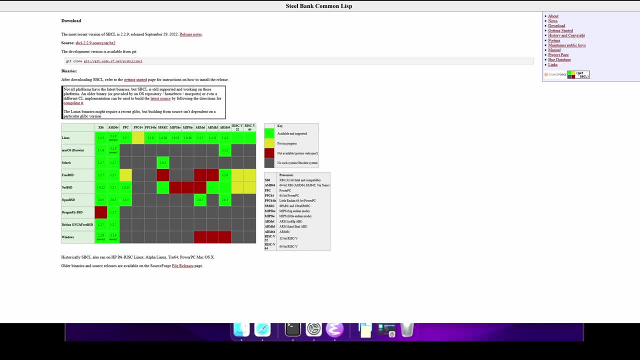 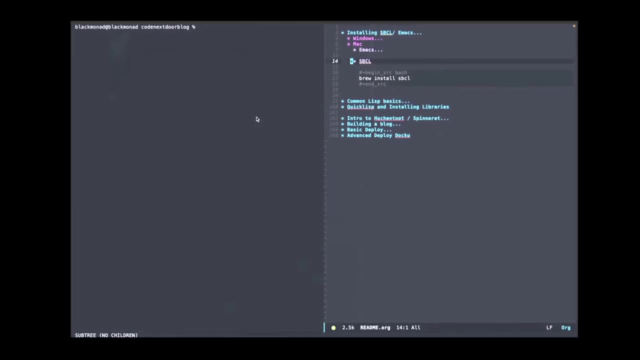 It looks like this spclorg, and they have a live binary for you to install here, or you can build it from source, whatever you like. Once you have a LISP installed, we will want to have some way of editing that. 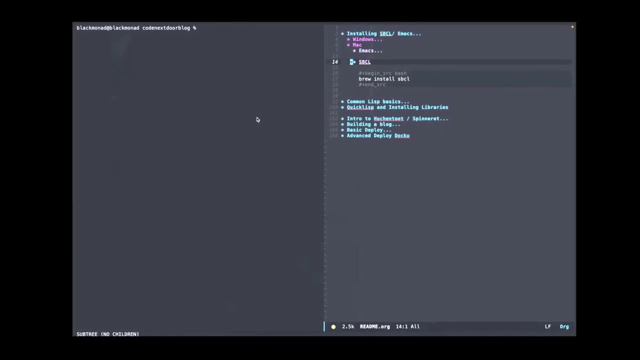 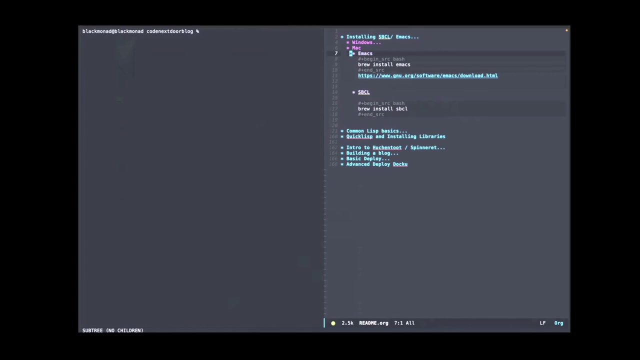 I highly recommend using Emacs. It has a bunch of cool features built in to work with LISP, like languages, and it's really awesome. So in order to do that, you can use brew as well: Brew, install Emacs, or you can build from source or download executables from GNU and the links. 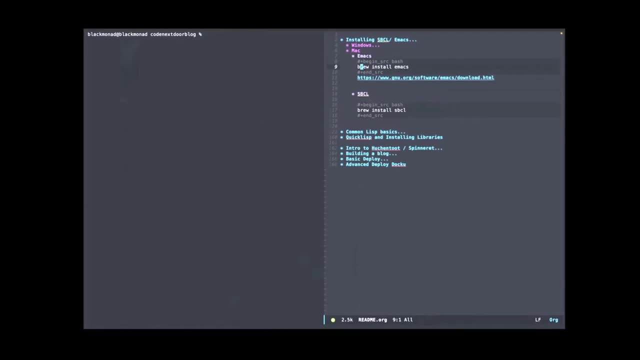 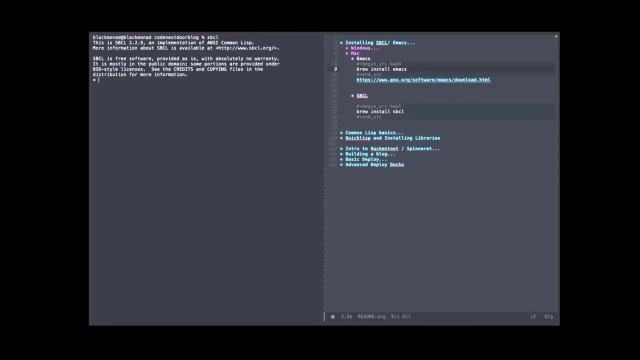 will be in the description. So, assuming you've gone through the steps and have installed SPCL and Emacs, start a terminal and let's just look at what SPCL has to offer. So we type in SPCL. this starts a REPL, A re-evaluate print loop type program, And I will start to go over the basics of. 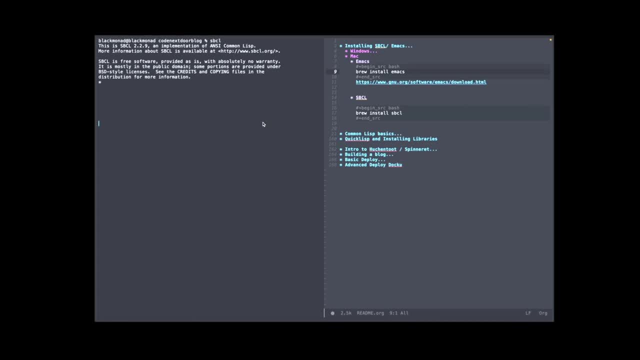 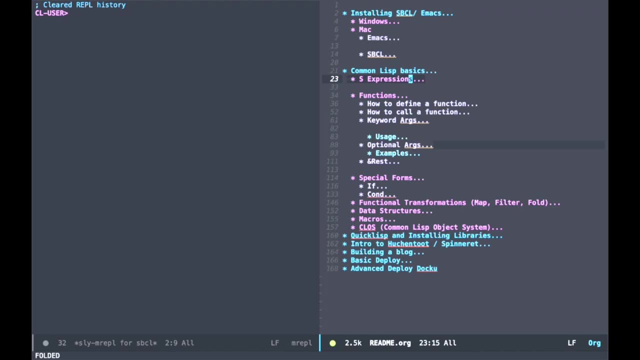 what LISP has to offer. and So in Lisp you essentially have two types of data: You have list and then you have atoms. Atom it can be a number, It can be a string, And a string in Lisp is just anything inside quotation marks. 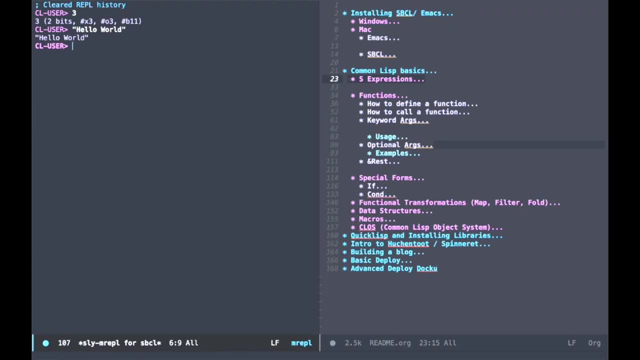 So, hello world, You can have binary And you can have hexadexal. Yeah, I don't know hex off the top of my head, But these are all atoms. And then the other thing you can have in Lisp are lists. 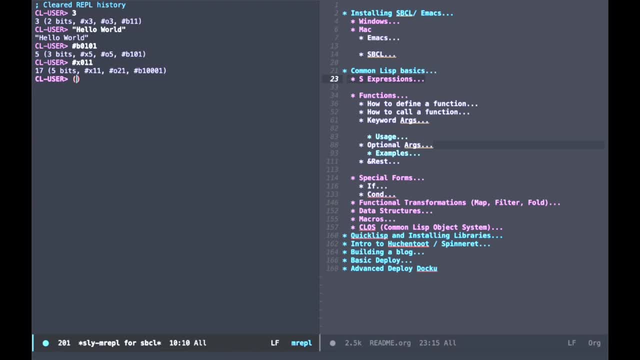 And in order to make a list, in Lisp you start with an open parenthesis and a closing parenthesis, And because I'm using Emacs, I have pair edit, which helps me write Parentheses faster, So you can put your atoms inside of your list. 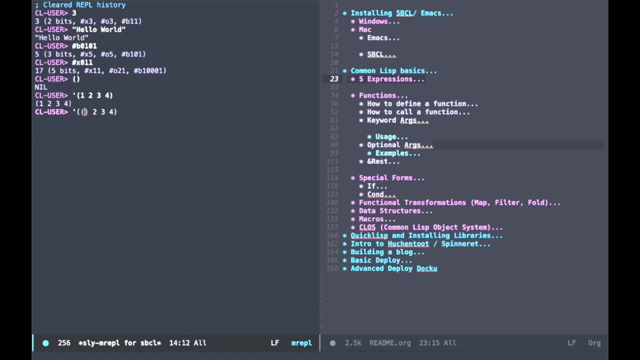 And you can have lists inside of your list. So you're probably wondering now: well, how do we do anything with these lists? So, in order to add things on Lisp, we'll cover that first, When you want to actually evaluate some expression. 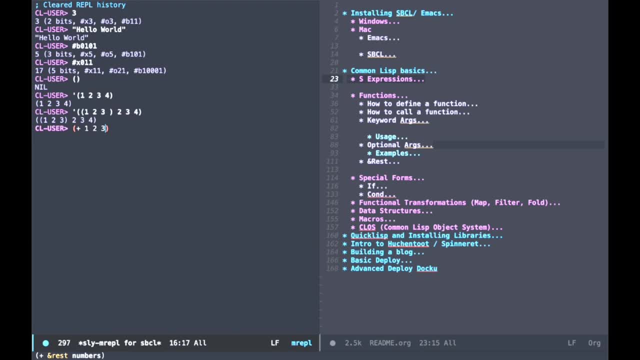 and not just have it represent the data. you write a list And this list is going to be special. The first thing in this list is going to be a function, And then every other element in this list is going to be arguments to that function. 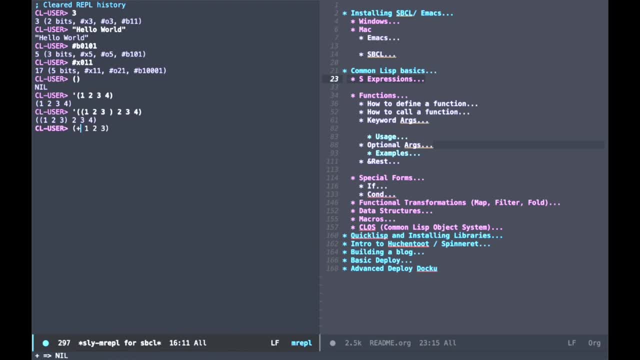 So here we have the addition function And we're passing it the arguments one, two and three, So we should see the result of six, which we do. So Lisp takes the first element of the list, treats that as a function name, looks up that function. 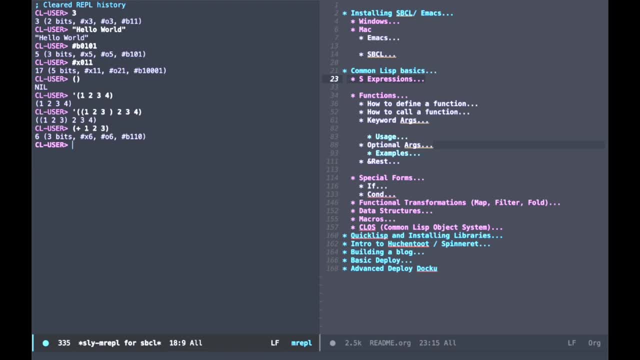 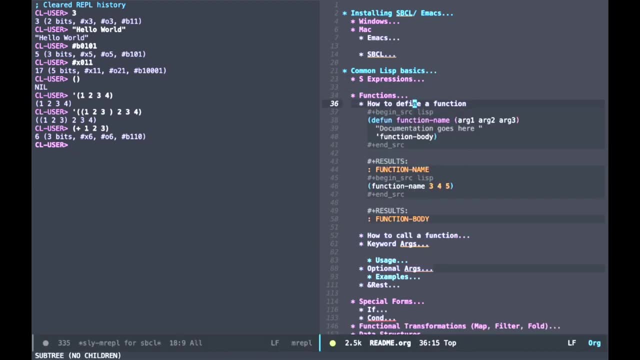 and then evaluates the rest of the elements of the list with that function. So how do we define functions? So how do we define functions? So how do we define functions? So you start off with a list which is just open parentheses, And then we use this word defund. 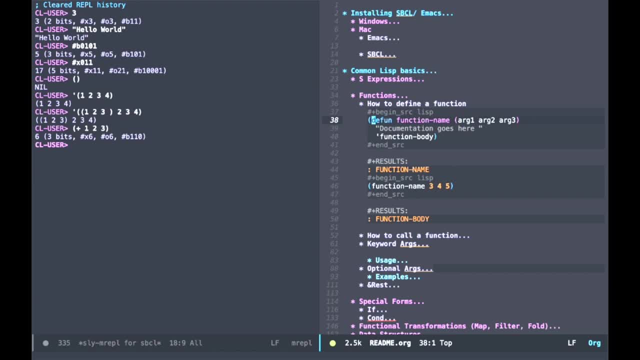 which you can kind of say stands for define function, And then we pass it as the second element in this list, the name of that function, And then, as the third element in the list, we pass it a list, And this list will contain all of the possible arguments. 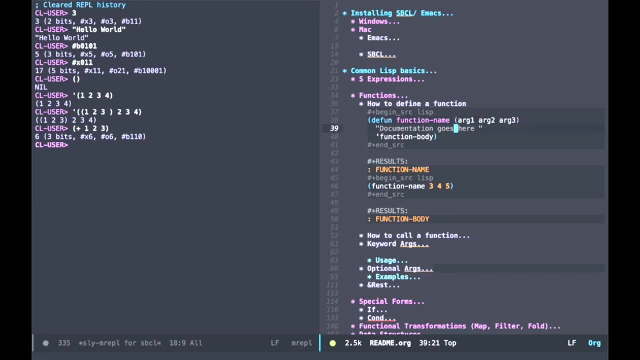 to the function name. The fourth element in the list is going to be a function name. The fourth element in the list is going to be a function name. The fifth element in the list is your documentation shrink, And this is essentially like how we document things. 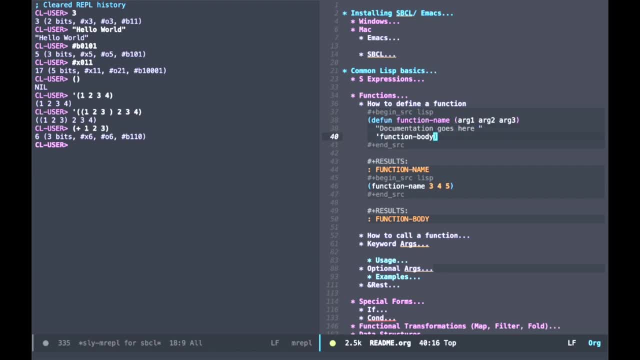 And then, finally, the fifth element is the actual body of your function. So if this is valid Lisp code and because I'm using Emacs, I can press Control-C, Control-C, and this automatically evaluates in my repo on the left, And this is sort of how people go about coding in Lisp. 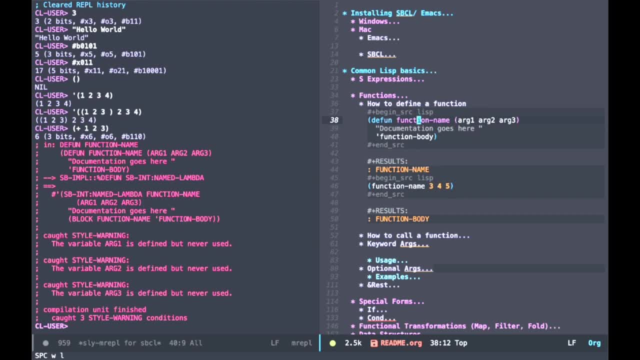 They write something and then they evaluate it and they write something else, evaluate it, and back and forth. And we already know how we use functions. We put them in the first position of the list and then we call them with their arguments. 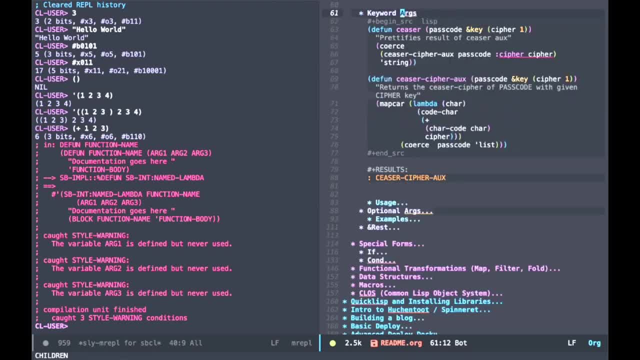 So list functions also accept keyword arguments. So say, we had like a Caesar cipher function and we want to essentially pass it some pass code to encrypt. And well, by default we want the cipher to be one, but we would like to offer to the user the option to pass in some other key. 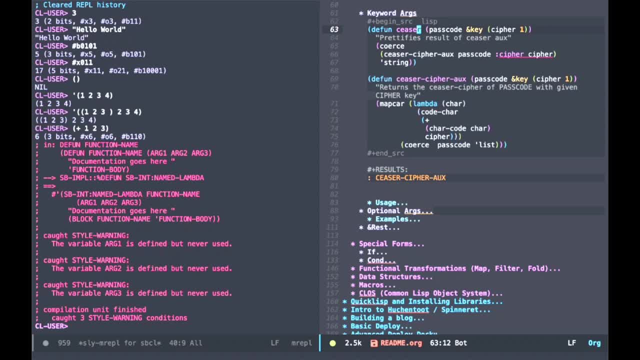 so they can like change the cipher to be something else. So Lisp offers the ability to define keyword arguments. So we have our first element, which is the defund special keyword, and the function name, Caesar in this case. Then we have the list of arguments that the function will take. 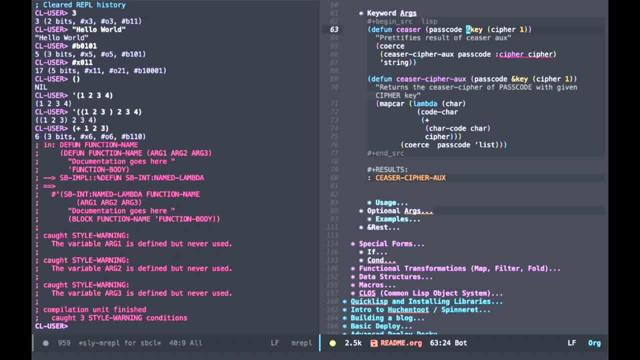 And this is a syntax- We're defining a keyword argument. So you did ampersand key and then a list of arguments and the default value for that argument. So if we compile this, Caesar and I come over here and use it. 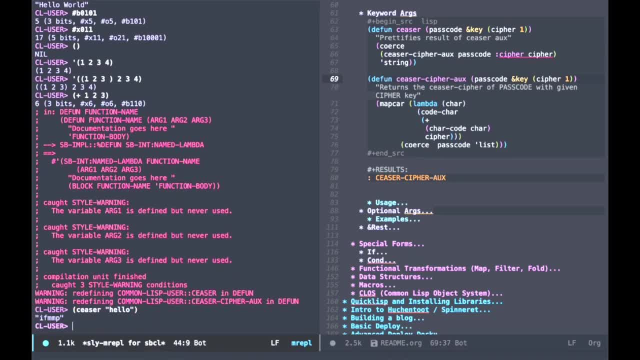 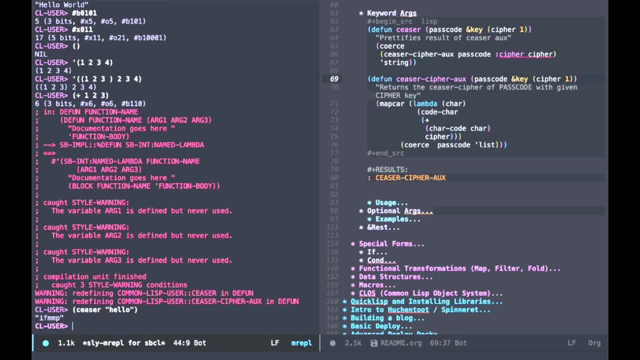 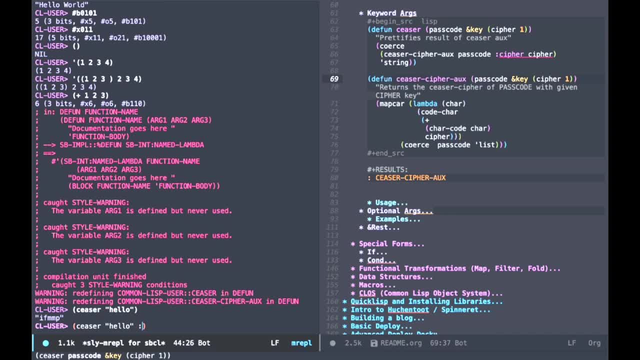 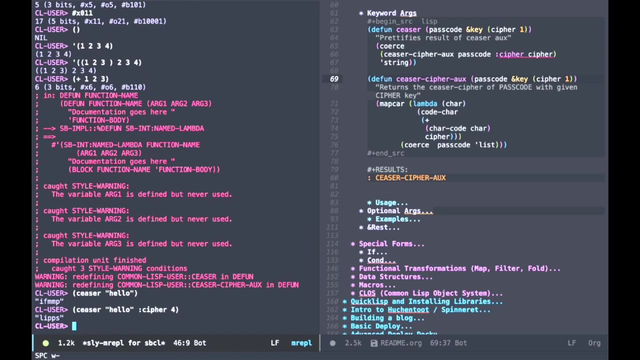 But say we wanted to define our key to be something else. So our key is called cipher, and then we pass it for, And now it's changing our key by four. So those are keyword arguments And similar keyword arguments. we also have optional arguments. 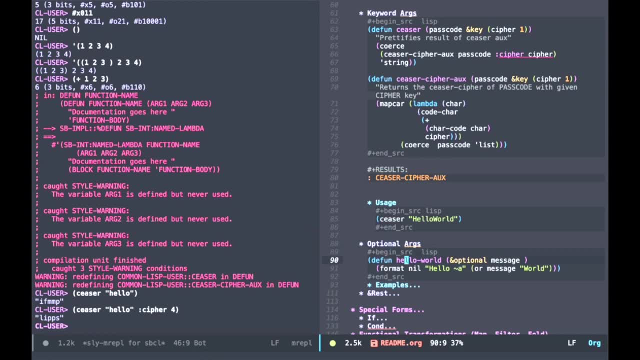 And these are arguments that we're going to use to do this, And these are arguments that we're going to use to do this, arguments that just don't necessarily have to be there. so, if you have the hello world function, here we have our list of args, and then we have the ampersand optional, and then 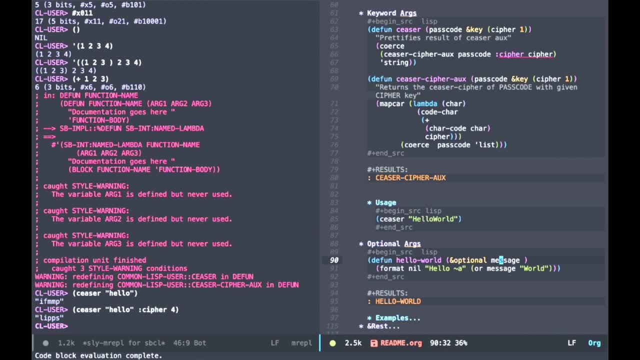 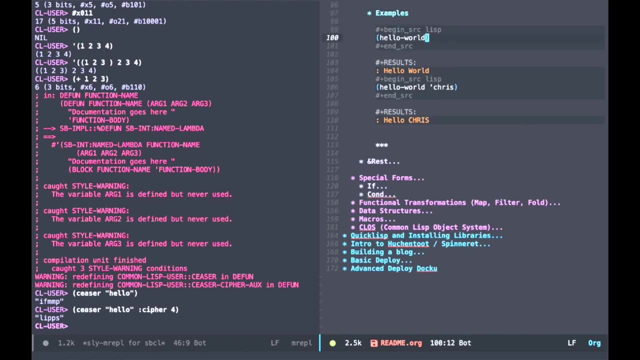 message is an optional argument that we can pass. so if we compile this by pressing ctrl c, now we have access to that hello world function. and let's run some examples. so if we just run hello world by itself, it prints out hello world. if we run hello world with chris- 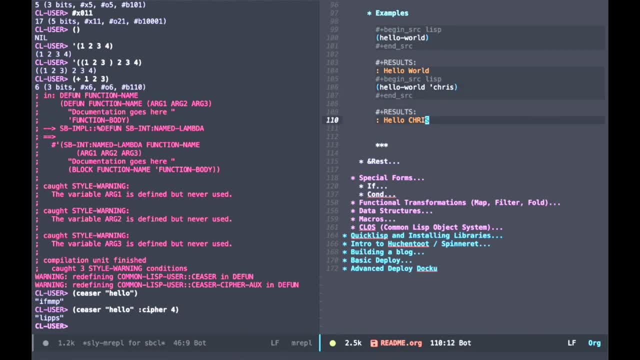 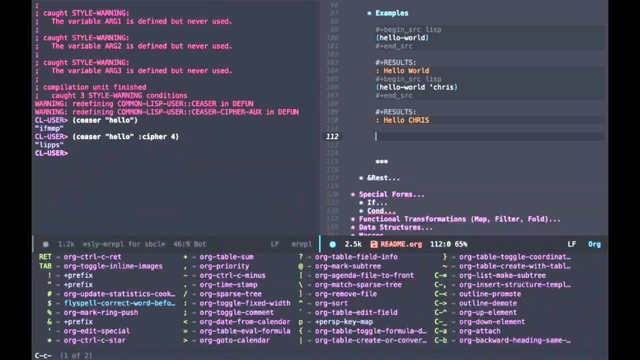 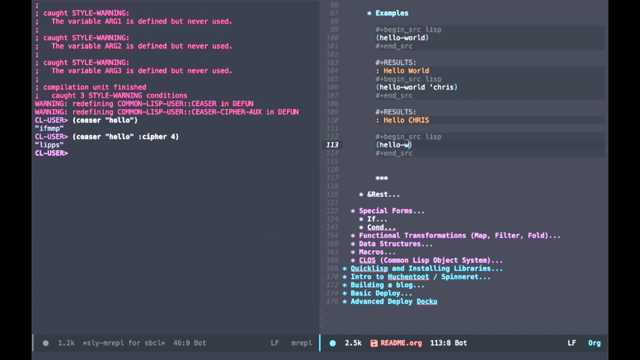 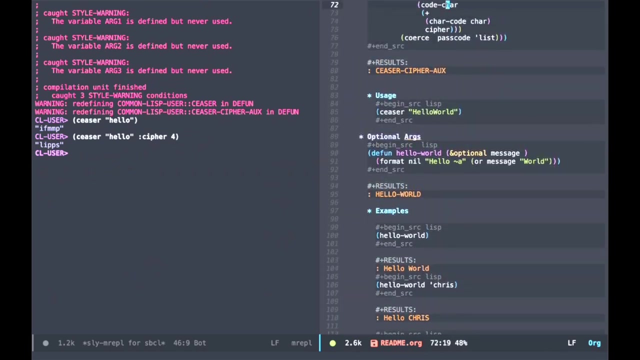 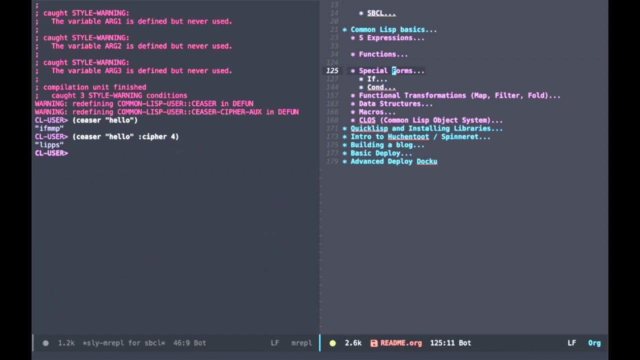 it prints out: uh, hello chris. and if we want another example here, hello world, andre, hello world. it prints out: hello andre. okay, so, um, that's how you define functions and lists, which i think is like the most important part of uh, a programming language. after that, um, i would say you have the. 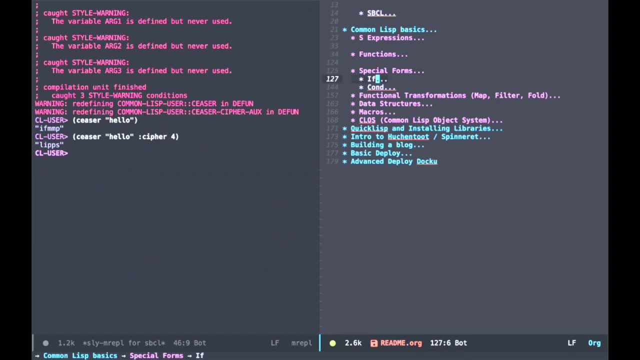 special forms of language. so you have like if statements and conditionals. so list has if statements. so in order to have an if statement, you write if and then the thing that you actually want to test your is if statement is going to be a conditional. so let's say, if we have an equal function. 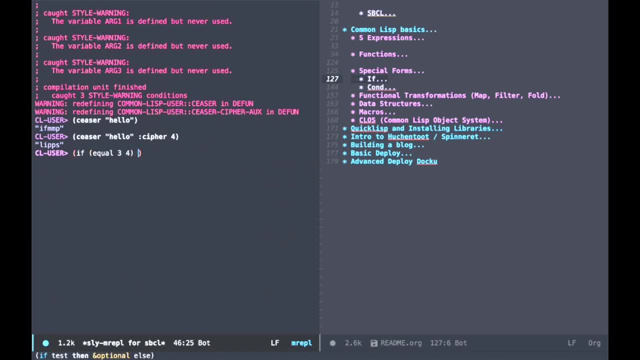 if three is equal to four, then we want to return nonsense, and if it's not equal to four, we want to return, uh, obvious. so this is statement is gonna clearly return obvious, right, because three does not equal. but that's how you do. a simple if statement: you have if in the the first position. 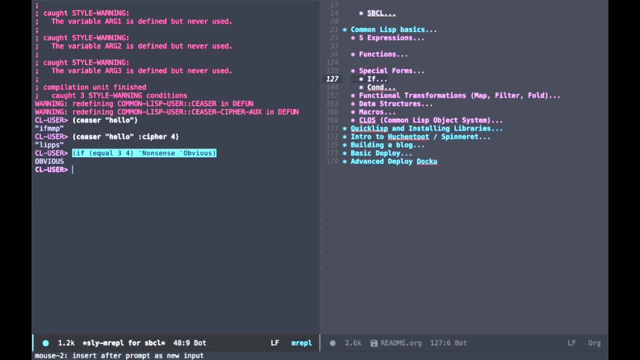 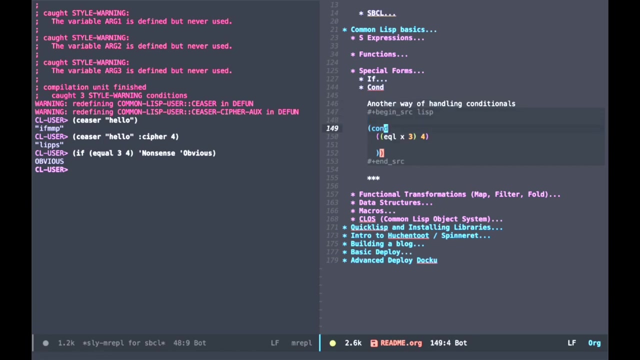 then you have your test and the second position, then you have your truth statement, like what happens if the statement is true? on the third position and the fourth position, you have the. what happens if the statement is false? now, uh, you might find yourself doing a lot of these types of if statements where, in other languages,